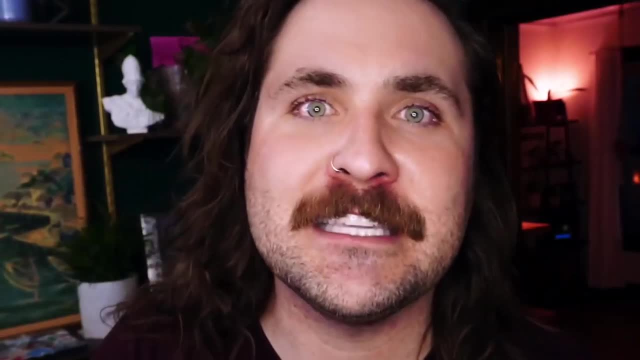 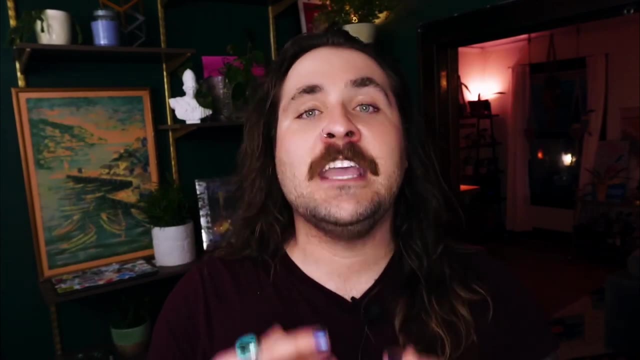 hopefully we can take you and bring you to the world of MongoDB schema design and taking advantage of all the cool features that you would not be able to do or use if you're using a relational database. There is a long history of research done on how to best split up data with relational database management. 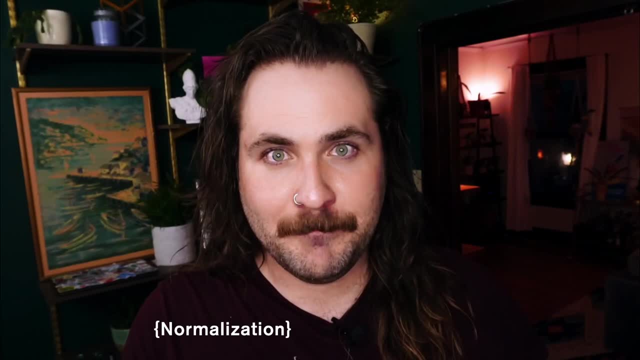 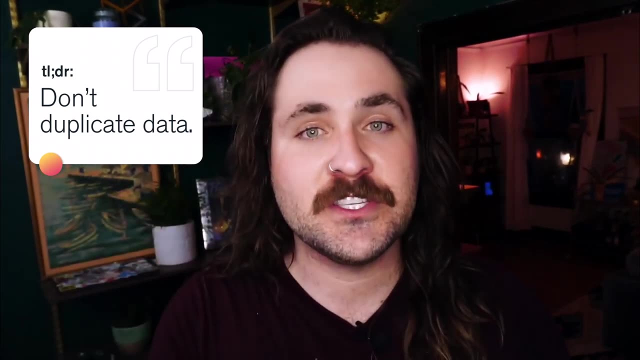 systems. If you're new to schema design, you're probably familiar with the systems And this process is called normalization. The TLDR of normalization is we're trying to split up our data into tables in order to reduce duplication of our data. Let's look at how we might model a user data in a 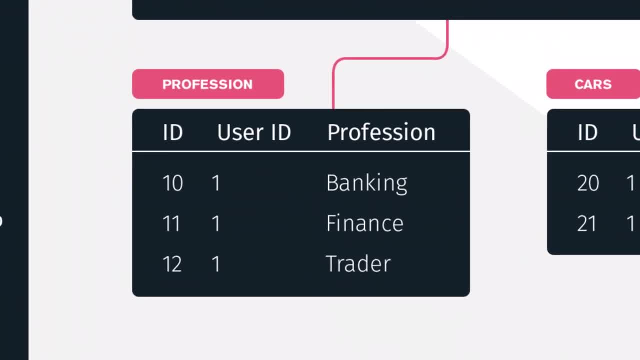 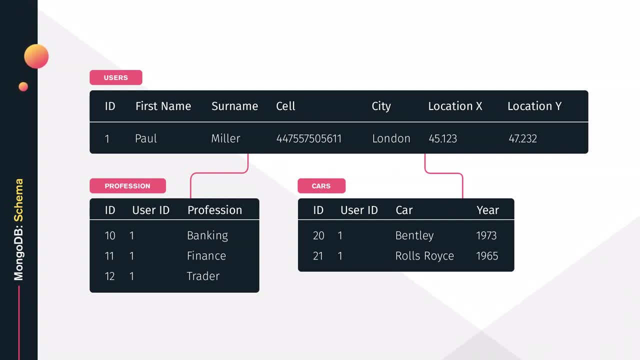 hypothetical application. So a user would have professions and cars we need to track with it. If we want to combine all that data together, we do something called a join on foreign keys And in this example you can see our user ID column in the professions and cars table is linking that data to the 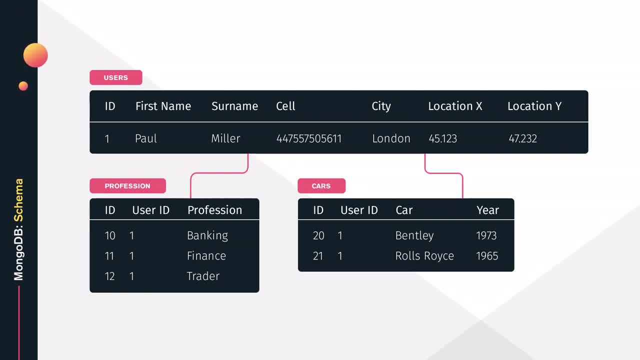 users table So we can run a query and pull all that data back together for us. So we're normalizing this data and we're able to do queries that join data sets together from separate tables. So we don't worry about duplication. So that's. 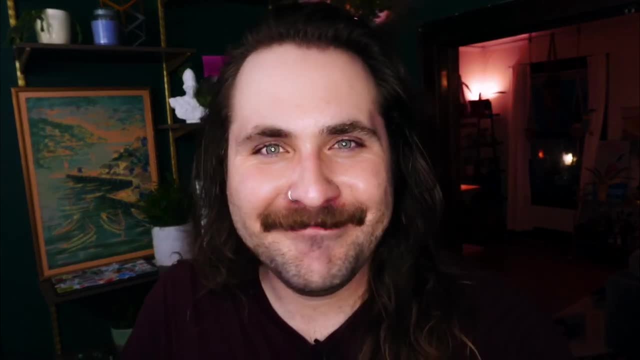 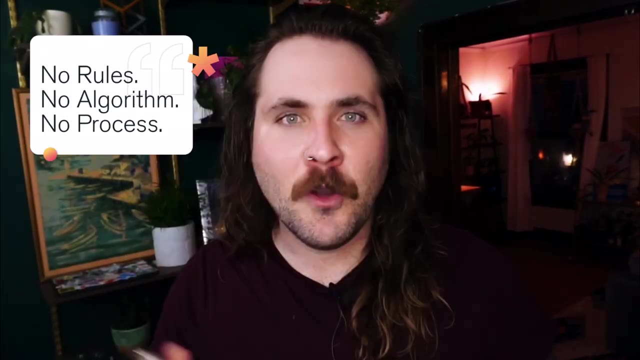 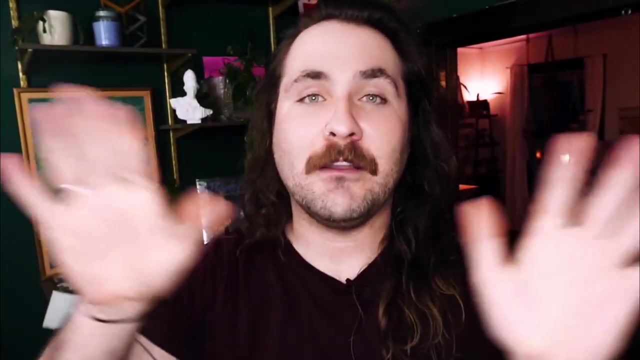 the super fast version of relational schema design. Let's look at MongoDB. Let's see what we can do with that one. MongoDB schema design is a little bit different: No more rulebook, No algorithms, No process, Nothing, Joe, what? How do we design a? 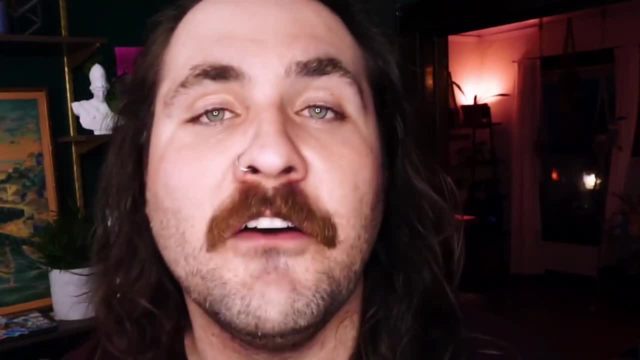 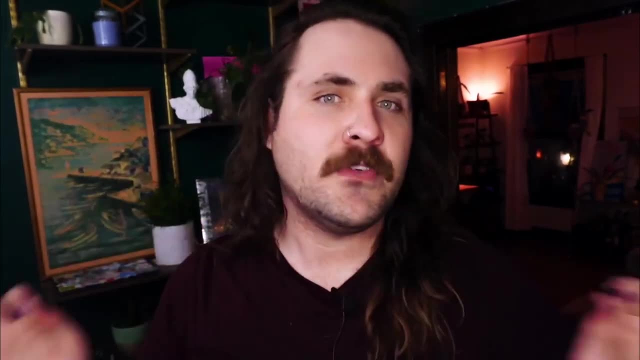 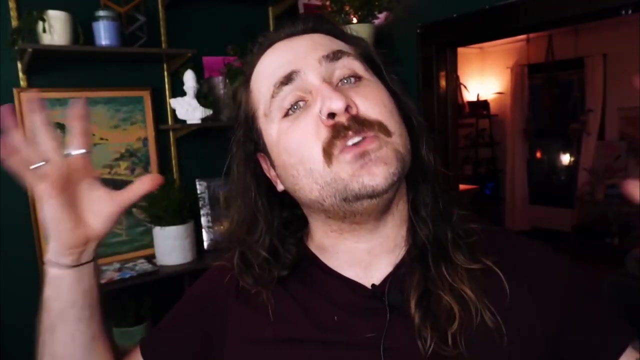 schema. if there's no rules, I'll tell you the platinum rule of MongoDB schema design: Design a schema based on the unique needs of your application. Nothing else matters. Two people might be dealing with the same data, but how that data gets used dictates how you want to design that schema. Let's take that user. 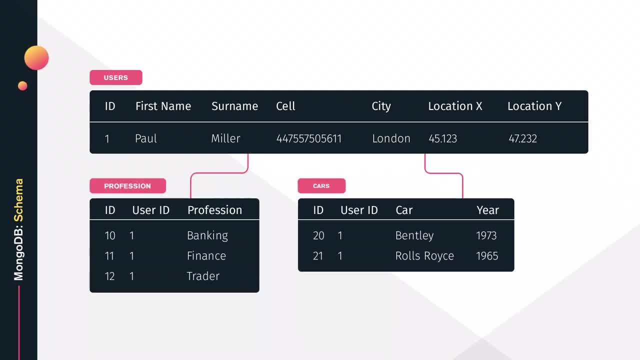 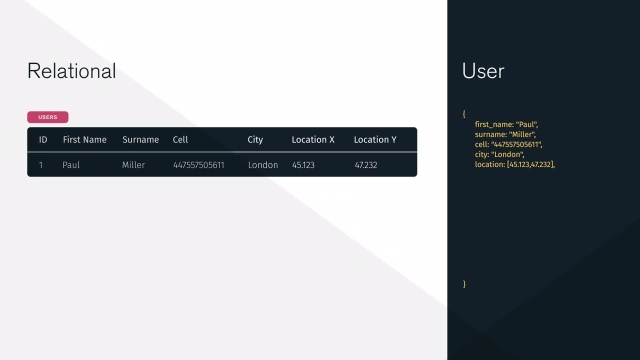 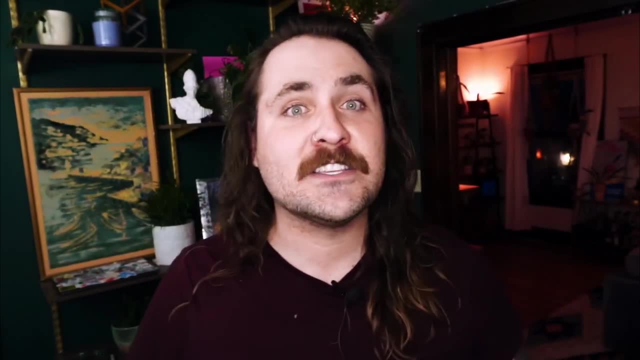 model That we were working with the relational table and let's convert that over to a MongoDB document. That first user table has a bunch of simple data in it that can just be reflected as key value pairs in a MongoDB document. The professions and cars table is a little bit different. Those have more complex data structure. 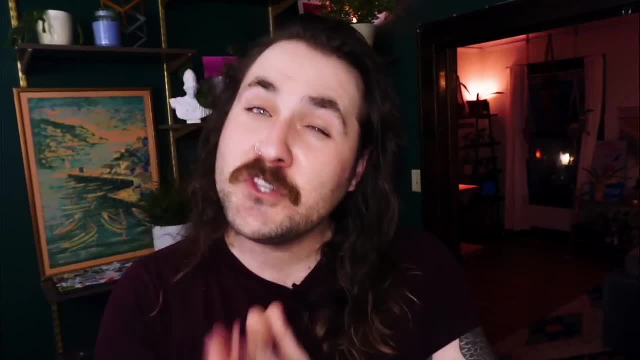 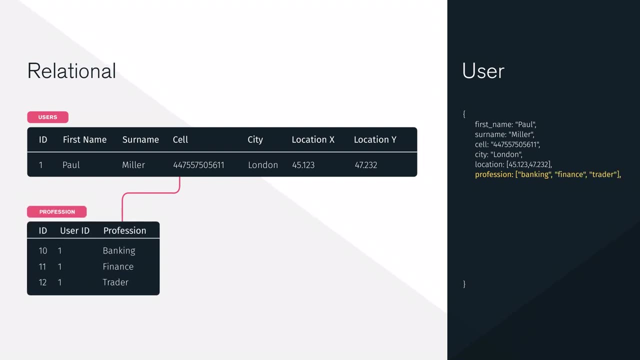 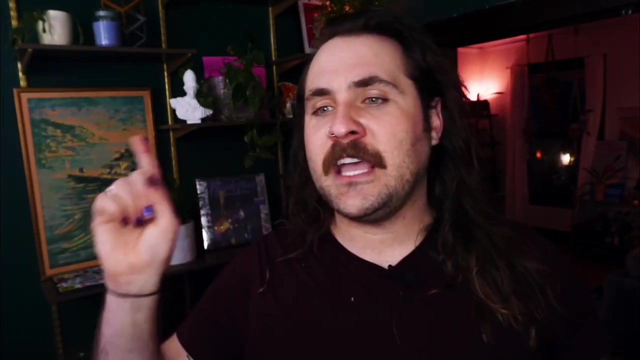 wanted to follow And that's hard to do in rows and columns but super easy to do. with MongoDB documents A user can have multiple professions and that's really easy to model with a document. We can just use an array of professions and embed that directly within that user document. Similarly with 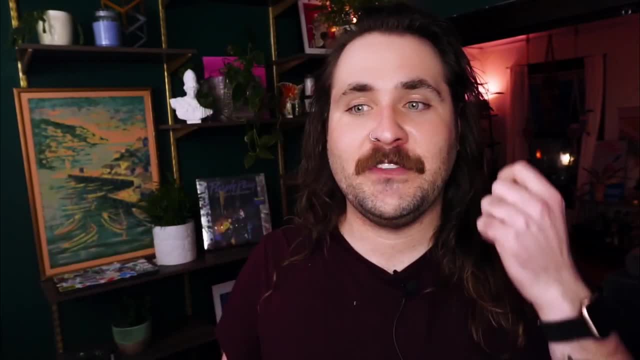 that cars table. it's very similar right, But there's more complex data structure. We have to keep track of both the model and the year for each vehicle, but we could just use an array of objects and embed that directly with that user. 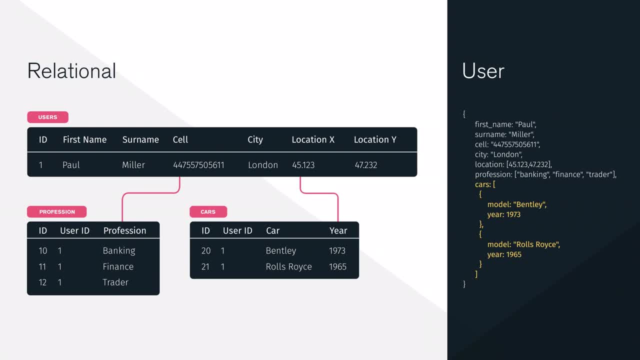 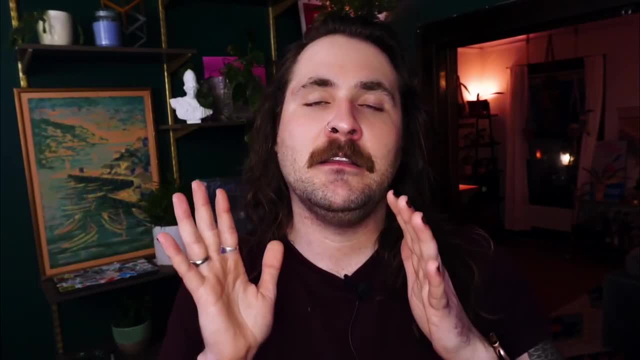 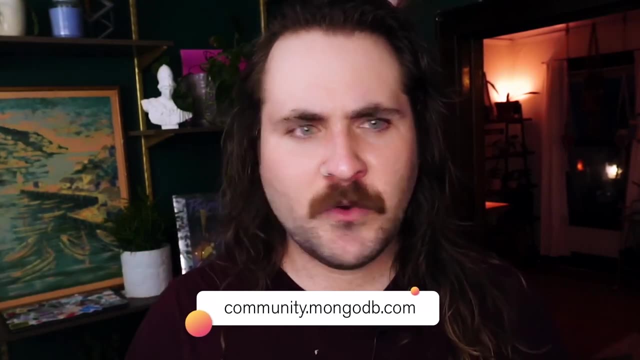 MongoDB. You can do that in MongoDB. You can do that in MongoDB. You can do that in MongoDB. The best place to do that is on the MongoDB community forums. Be sure to check out communitymongodbcomm and let me know what your questions are. Yeah, I'd love to take a look at. 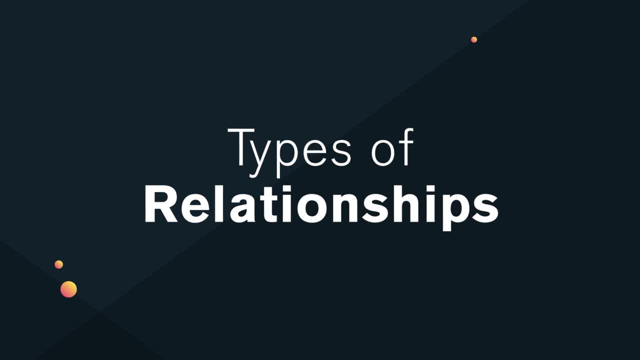 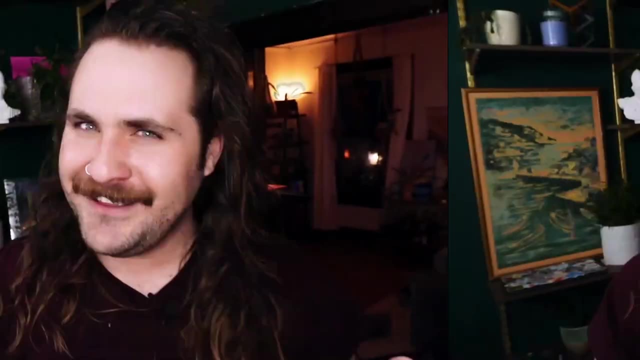 them. There's a link in the description below. Now let's discuss types of relationships and how we would model those with MongoDB. First one we're going to cover is one-to-one. One-to-one makes me think about going to Target. Do you know how Target has those frozen meals for one? 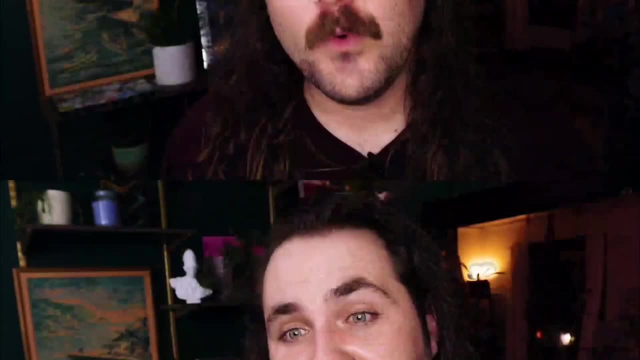 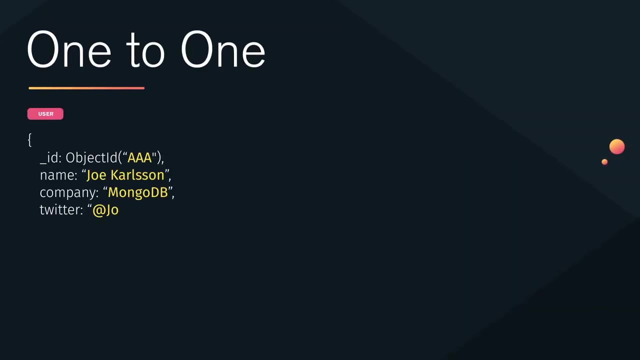 One Joe equals one meal for one. that's it. They're delicious. One-to-one relationships in schema design are very similar. actually. One user has one name, one company, one Twitter handle, one Twitch handle, one TikTok, one website. one-to-one. 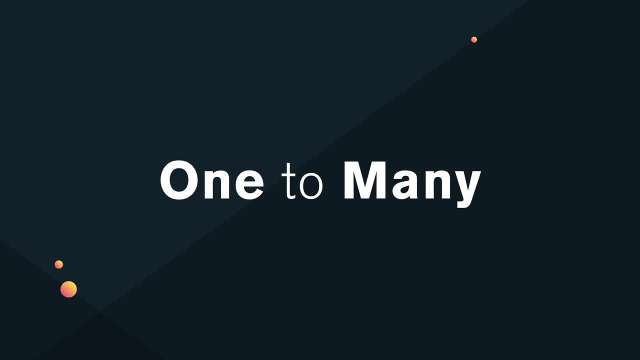 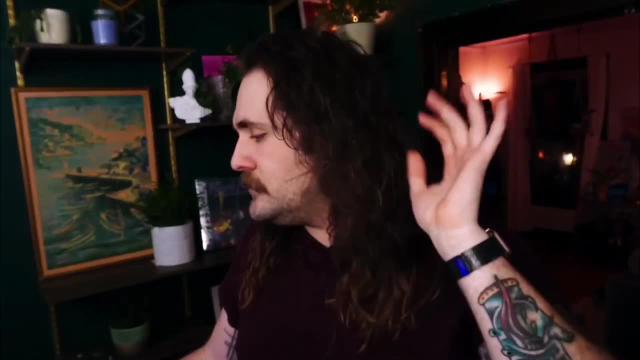 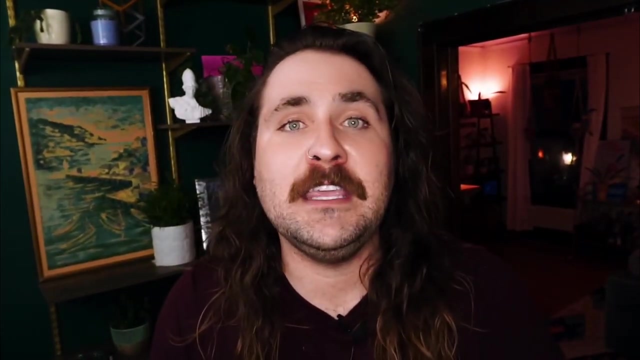 Let's take a look at one-to-many. One developer might have many stickers on their laptop. One me many developer stickers. Let's say, for example, you are asked by your boss to build an e-commerce store. We need to be tracking all of. 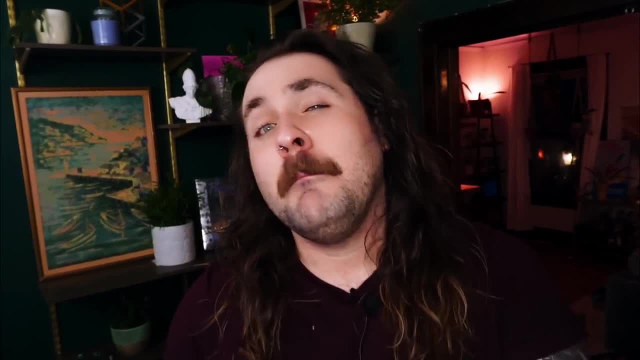 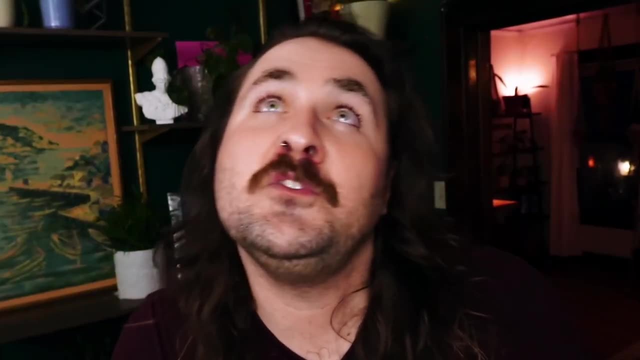 the products we're going to be selling in a MongoDB database, But we also need to keep track of all the parts associated with each product in our catalog. In this situation, let's assume that we don't need to access all of the subpart information often. 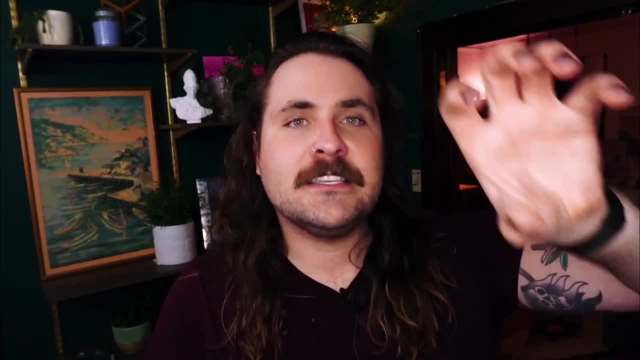 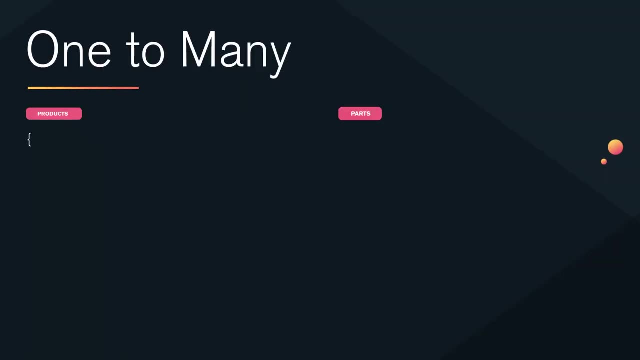 So let's pull that out, let's separate it. We have a product document. that's all the metadata, but we also want to keep track of that relationship. So we have a parts array within that document and that would have object IDs that link us to. 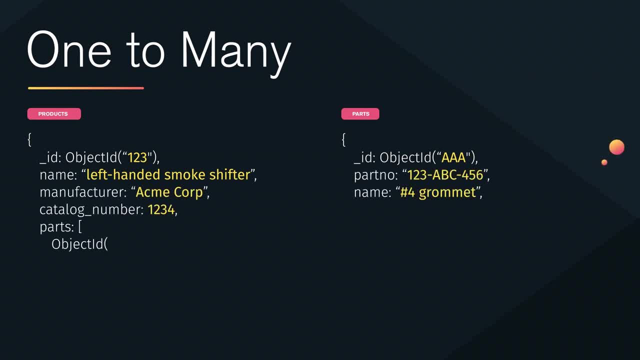 all of the other parts documents within our same collection. We could run queries then that would be able to go and pull all of the associated object IDs and we get all that data together. But if you don't need it very often, let's pull it out, no problem. 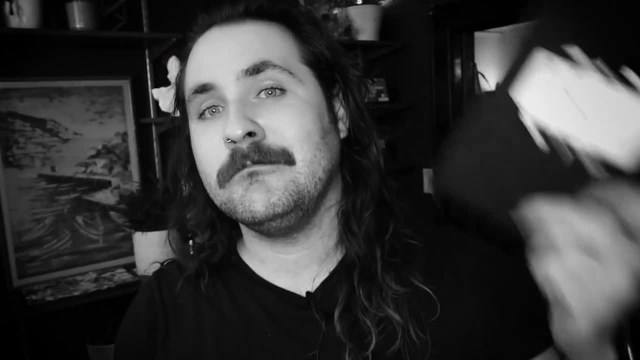 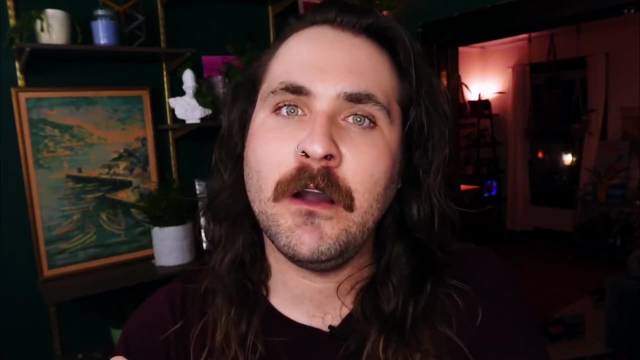 Do you remember when I told you that we threw out the rule book? Remember that I lied. I made up some rules to help you, dear watcher of this video, design scalable schemas for your application. My first rule: I favor embedding. 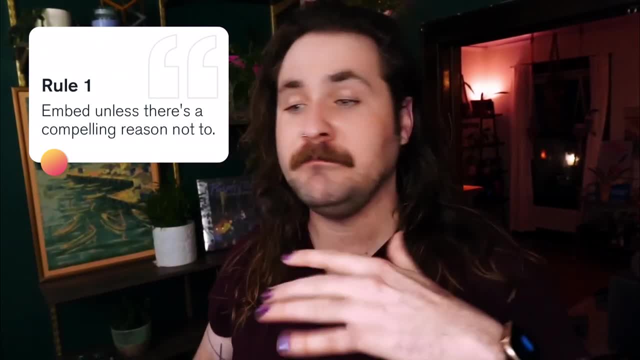 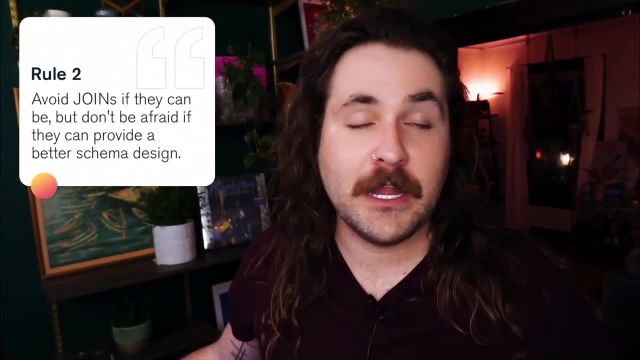 unless I have a compelling reason not to embed that data. Just look at this one-to-many relationship. Rule number two is also related. Avoid joins if they can be avoided, but don't be afraid to use them if they make your schema design better. 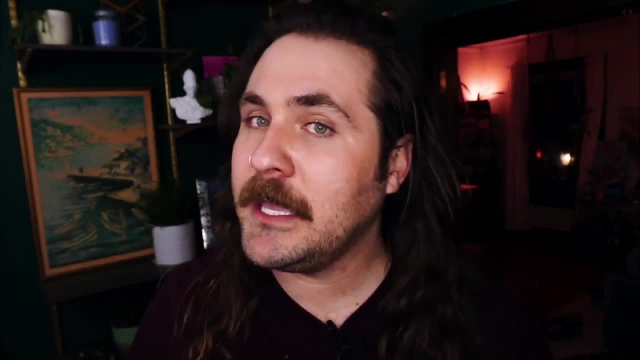 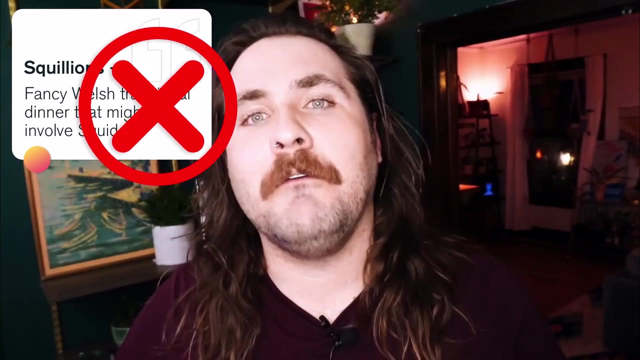 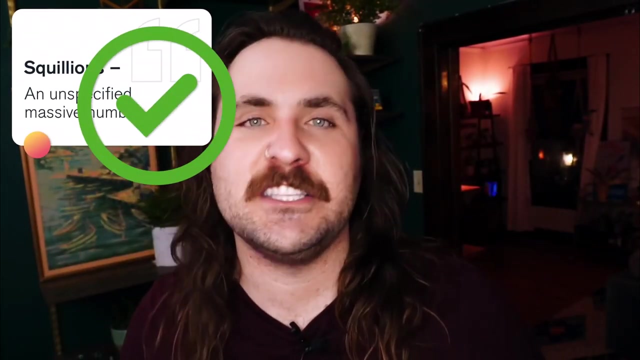 Squillions is in fact a real word. I did not make it up. Squillions sounds like a fancy Welsh traditional dinner that might involve squid in some way. Squillions actually means it's a unspecified massive number. Just think million, zillion, gazillion. 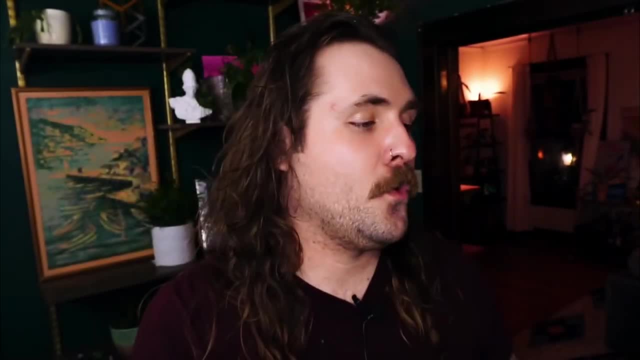 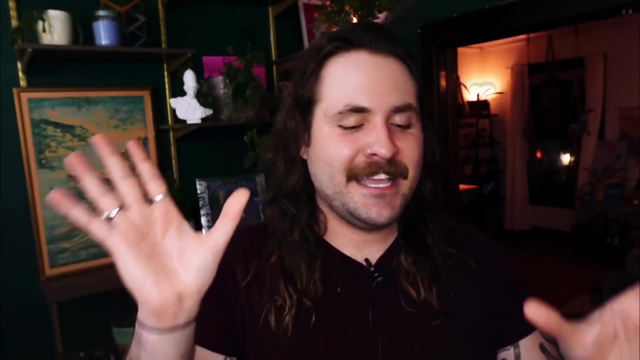 Imagine with me, if you will. you've been asked to build an application for logging. I'm not talking about timber logs. I'm not talking about lumberjacks. What I'm talking about is server logs. We could potentially be generating a squillion number of events. 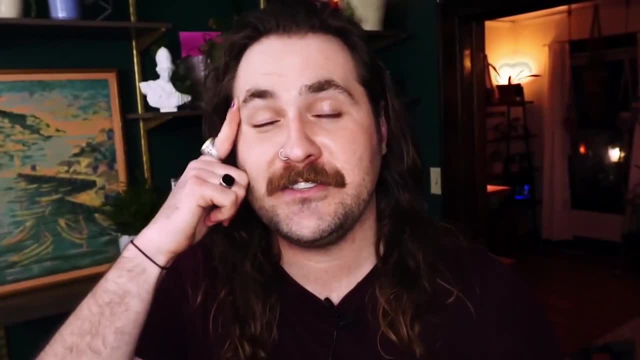 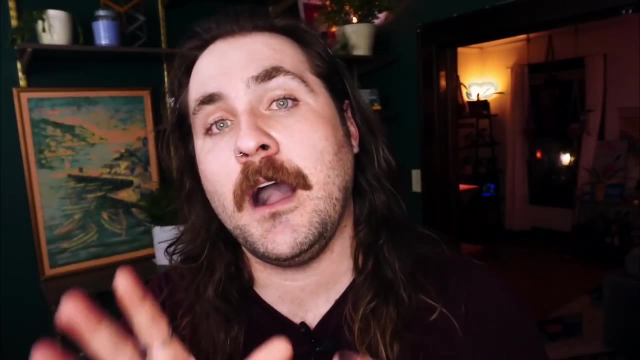 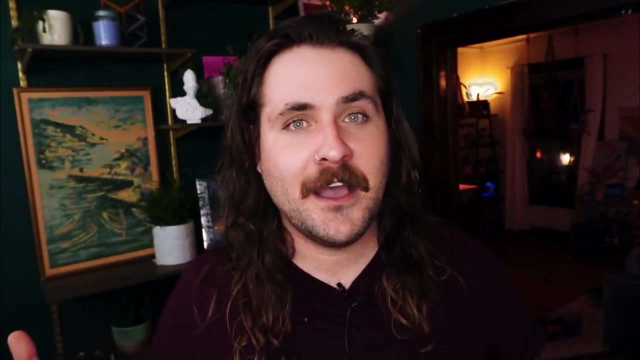 they're just keep tracking everything that happens on these servers for years and years and years. The issue that we come into with this schema is that there is a 16 megabyte per document limit on a MongoDB document If you have an array of object IDs and you're blogging massive amounts of events. 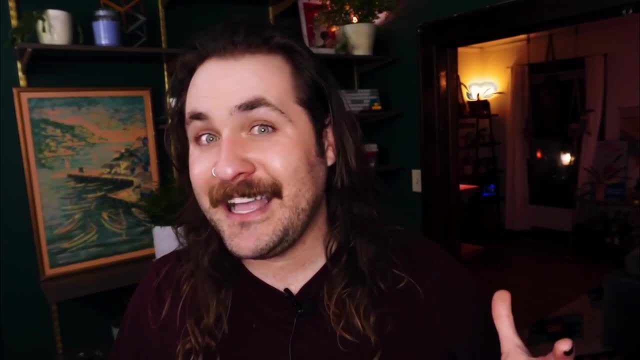 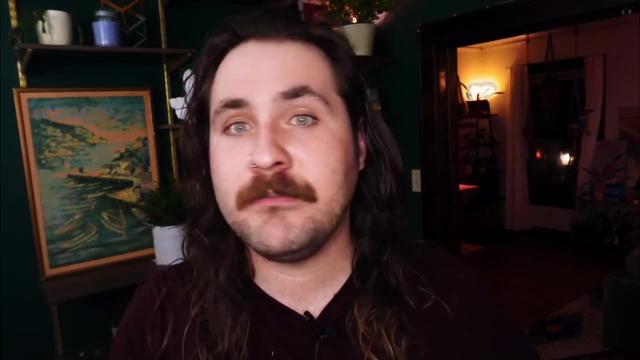 eventually, you're going to hit that 16 megabyte per document limit and that's going to break your application, which we don't want. We want to make sure we're designing a schema that can handle infinite growth on some factor or some sector or application. 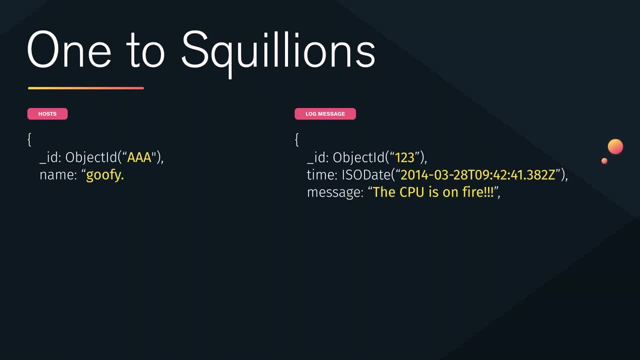 For this example, we're going to have a host document and then for each log event on each of our servers, we're going to generate a brand new MongoDB document. Each of these log messages will be responsible for tracking the host or the source server that the messages are from. 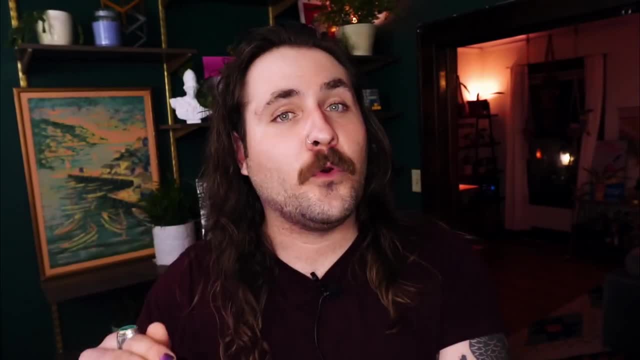 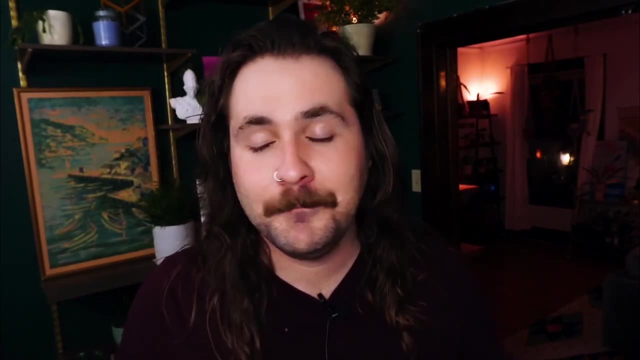 If we keep track of it with this reverse reference, we don't have to worry about having an array that grows an unbounded size and it might potentially hit that 16 megabyte per document limit. Rule number three: arrays should never grow without bound. 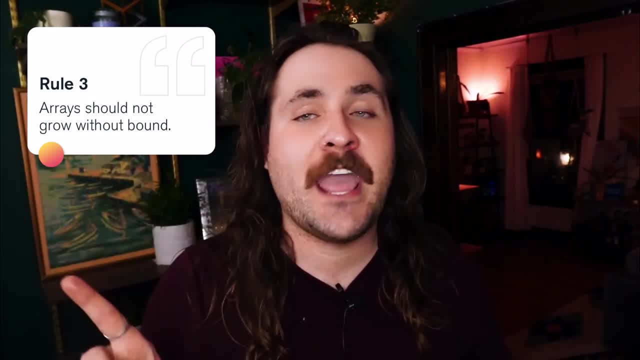 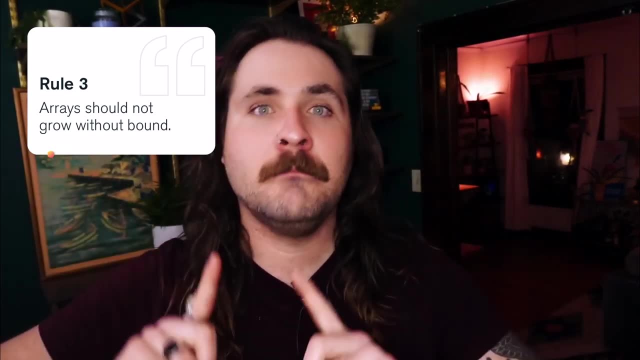 If I ever see a schema design that potentially could have an unbounded growth within an array, that's a massive red flag for me that we need to readdress and reconsider the schema design for that application. Let's imagine that you are building a to-do list. 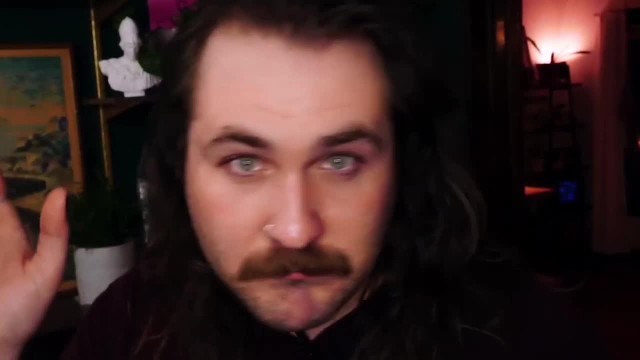 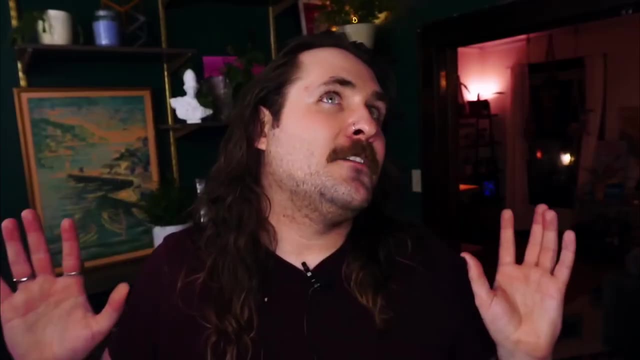 Each user in our application could have many to-do items on this to-do list, but also a single to-do item can be owned by many users. We're going to be taking lessons from all of our previous schema design relationships and apply them here. 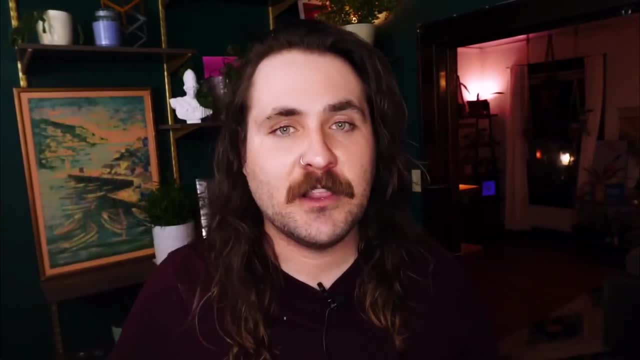 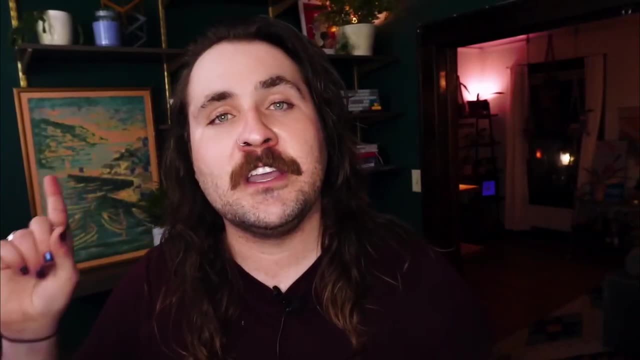 We would have user and to-do item documents within the same collection and users would have an array of object IDs that associate with the to-do items they own. But we're also going to need to track the multiple owners and we're going to be doing that on the to-do items. 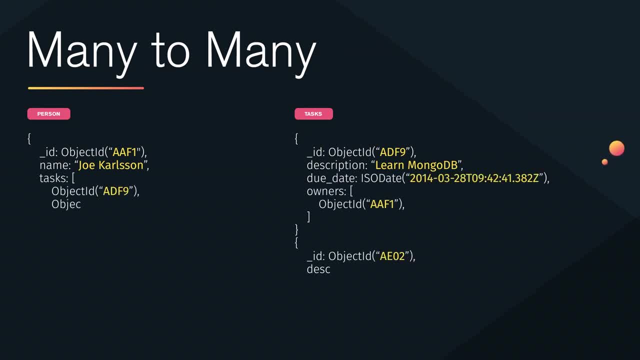 On the to-do item. they also have a reference to an array of object IDs of the owners who are working on that ticket. We have a reverse reference that two-way relationship is being maintained and we can write queries that can pull all that data out for application. 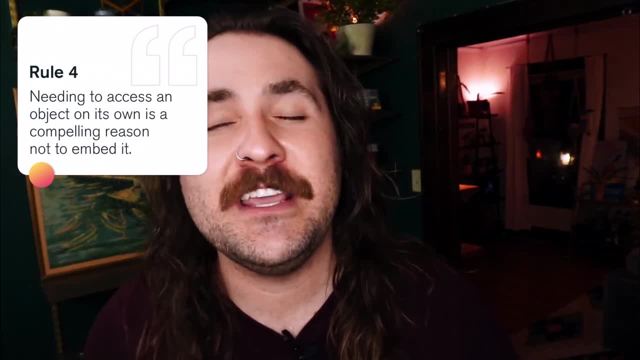 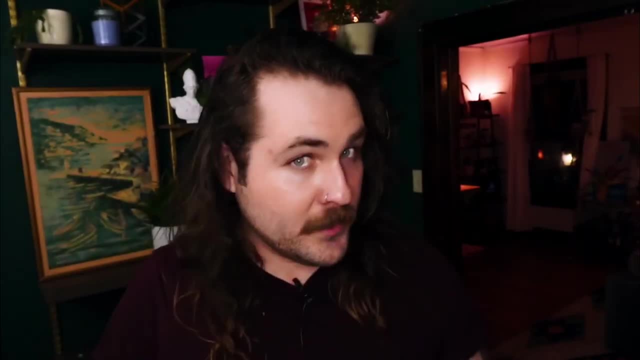 Rule number four: needing to access data on its own is a compelling reason to not embed it. That also leads me to rule number five, the platinum rule. Do you remember what it is? Design a schema based on the unique needs of your application. 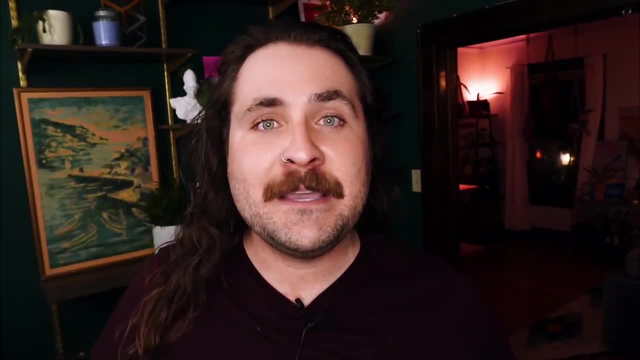 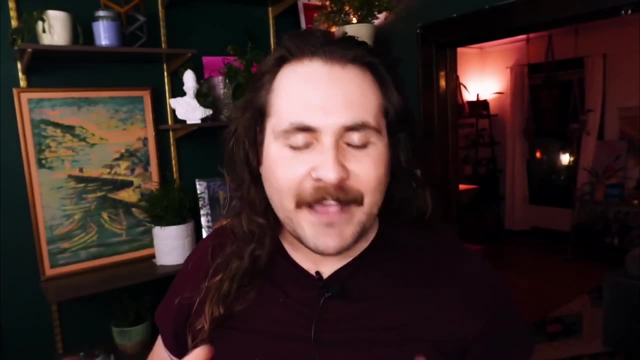 That's the only thing that matters. We've covered MongoDB schema design and a bunch of the basics here today. If you want to get better at MongoDB schema design, what's the best way to do that? I think videos are a great place to start. 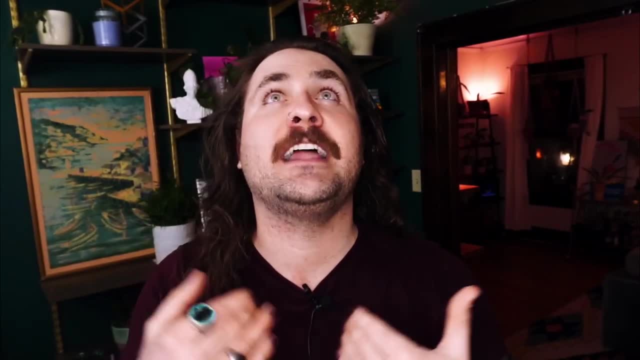 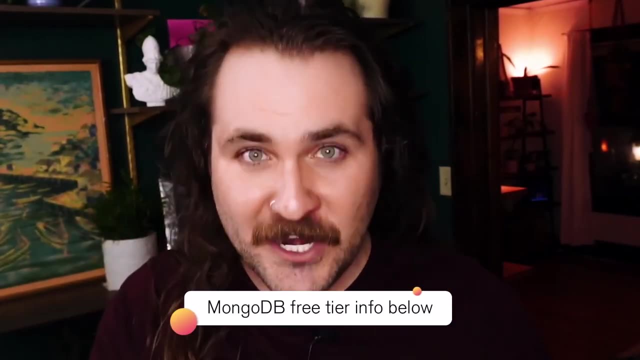 but for me to truly grok a subject, I need to make sure that I am actually doing it and playing with it and trying it out. The best way to do that is to sign up for the free tier of MongoDB Atlas Link in the description below. 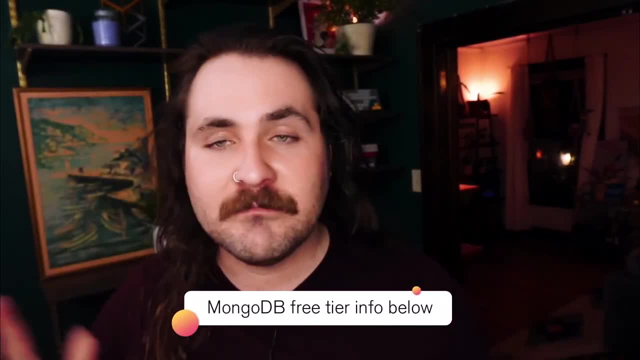 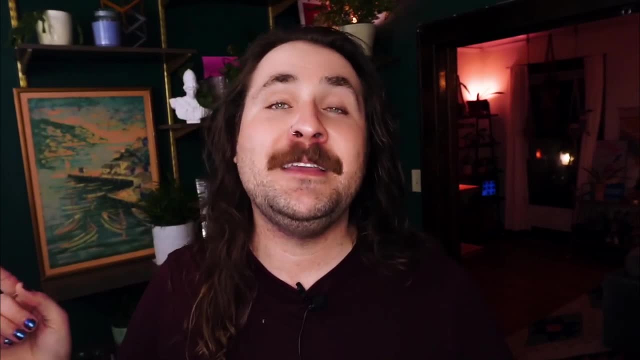 It's free. There's no trial period. As long as you're under the data cap, you're fine. It's amazing. You should check out my colleague, Lauren Schaefer. She did an amazing series on MongoDB design anti-patterns. 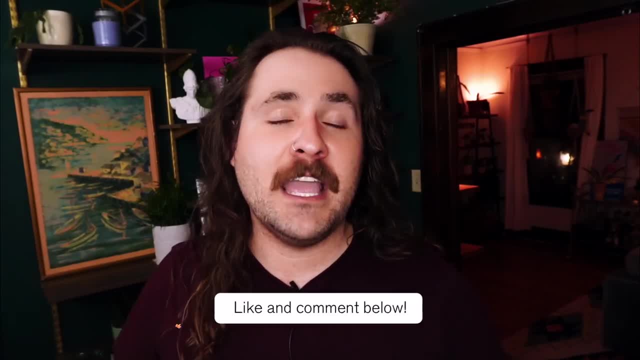 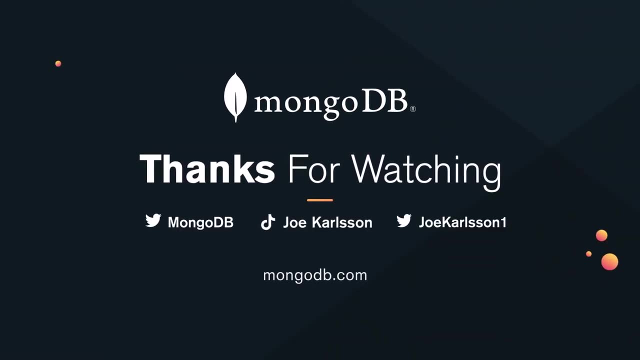 which tells you what not to do: Link in the description below. Be sure to like, comment and follow for more content like this. Let us know We'd love to make more for you.